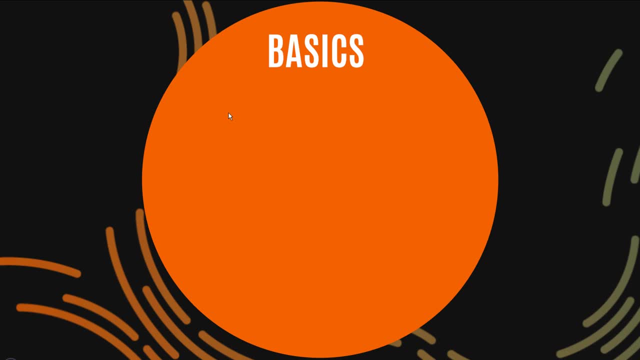 Anyway, the basics are pretty straightforward. Now I'm going to first throw some formula and symbols at you and then we'll try to find. then we'll try to calculate a mean from an actual sample. But in statistics we have this pronumeral x bar which we use to describe a sample's. 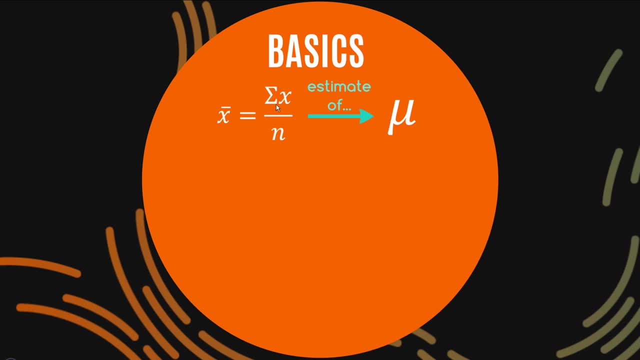 mean. And to calculate the sample's mean, it's going to be the sum of x. This big Greek symbol, here sigma, indicates that we are to sum this particular variable, And then we divide by the number of observations, which is n. 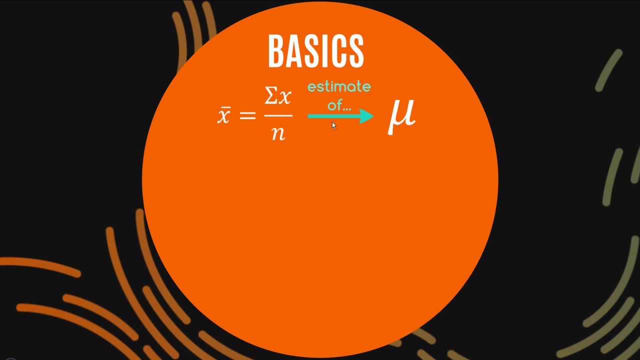 And in doing so we calculate x, bar, And that provides us an estimate of this Greek letter mu, which represents the population mean. So that's the whole principle behind statistics: We have a sample. we can create a statistic from that sample, in this case a sample mean. 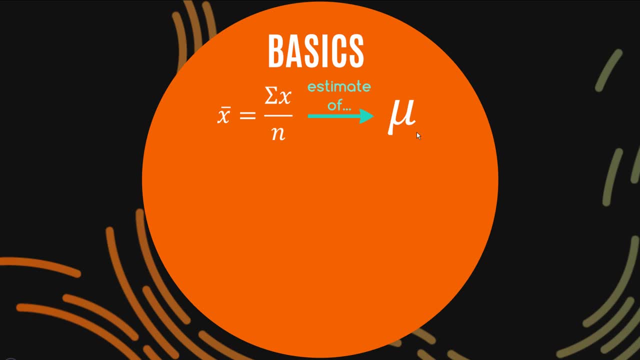 And that sample mean is an estimate of the true unknowable population mean. So, for example, if we're to find the average height of professional basketball players using this following random sample, you can see we have five players in our sample, each of their heights given here, and we can use that formula fairly straightforward: sum. 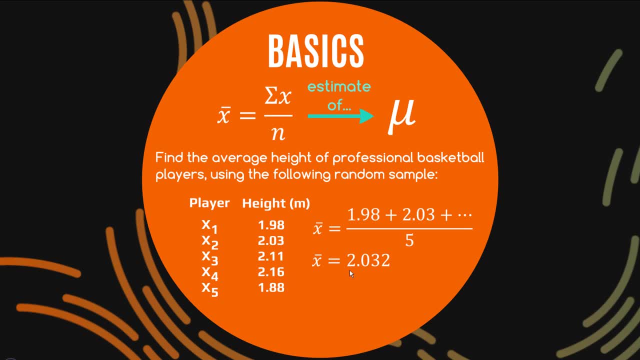 everything up, divide by five and we find that the average height in the sample x bar is 2.032.. Now the point I was making above here when I say it's an estimate of mu, Is to say that this is our best guess now as to the true average height of professional. 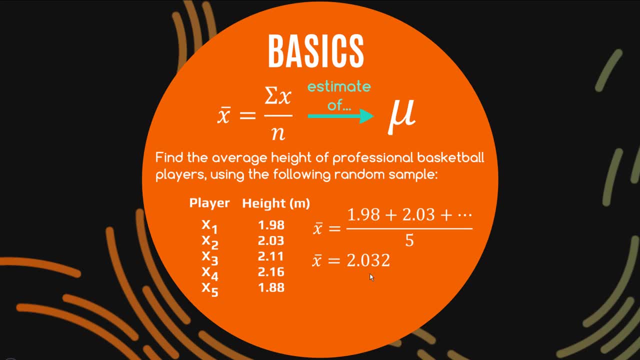 basketball players. They seem to be, on average, 2.03 meters tall, which is bloody tall, But appreciate that this is actually an arithmetic mean. We've just called it a mean so far, but there are other types of means that we're about. 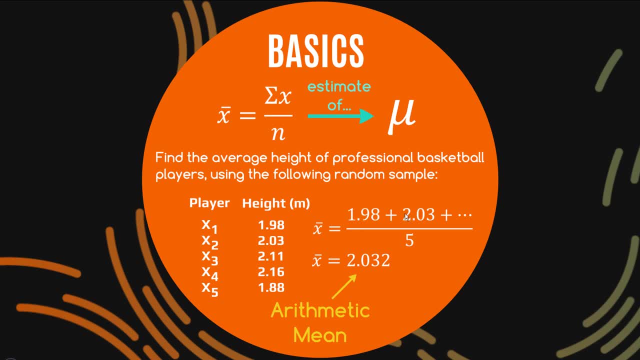 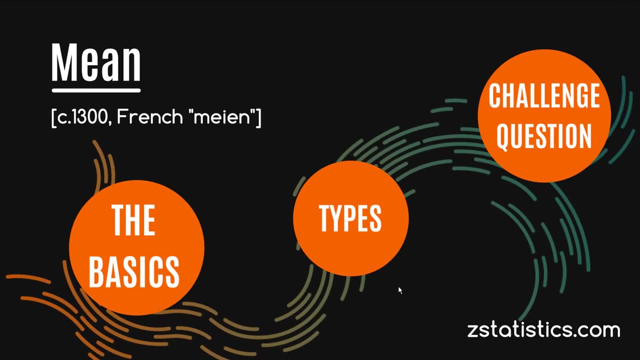 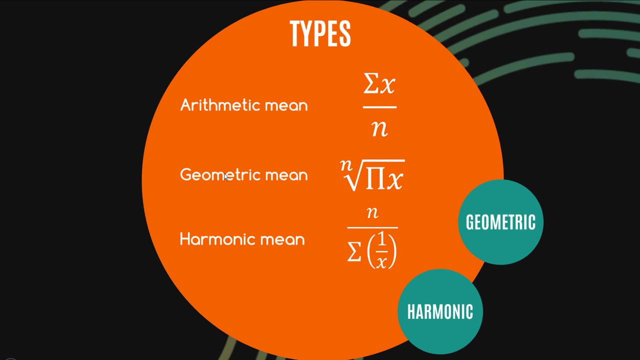 to be introduced to, And this one, where we just add up all the observations And divide by n, Is called the arithmetic mean. So let's have a look at some of the other types of means. So here's our arithmetic mean again. 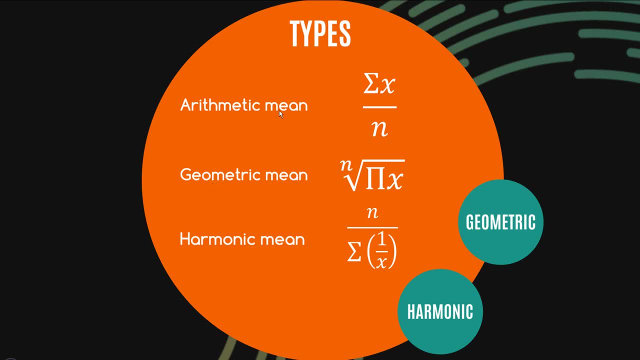 There's also something called a geometric mean which, unlike the arithmetic mean, you actually need to find the product of all the observations in the sample and then take the nth root of that product And we'll see how that works in just a second. 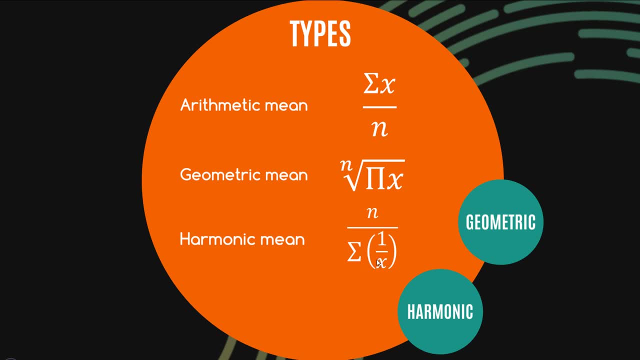 A harmonic mean is quite interesting too. What you do there is you actually invert all the observations. You can see we've got one on x here. all those are being summed together. You invert all of the observations, then find the average of all the inverted observations. 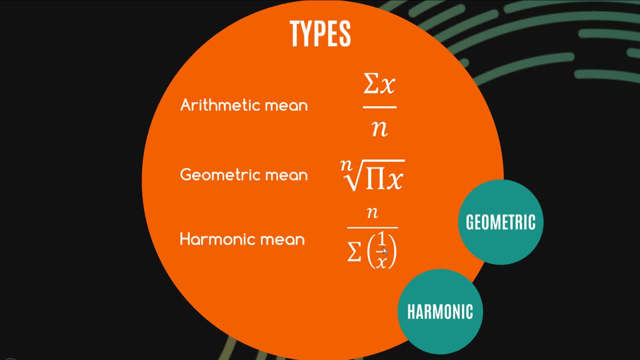 And finally you invert back that average. But look, in reality you're going to be dealing with the arithmetic mean 99% of the time, But in certain circumstances these do pop up and they're actually more interesting, if you ask me. 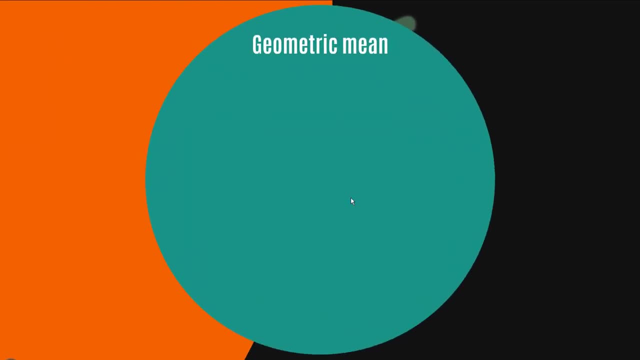 Hence why I'd like to focus on them. So let's have a look. What's a geometric mean? Now, this example will show you where the geometric mean actually gets its name from: Geometry. funnily enough, A rectangle has dimensions 9 meters by 4 meters. it's a pretty big rectangle. 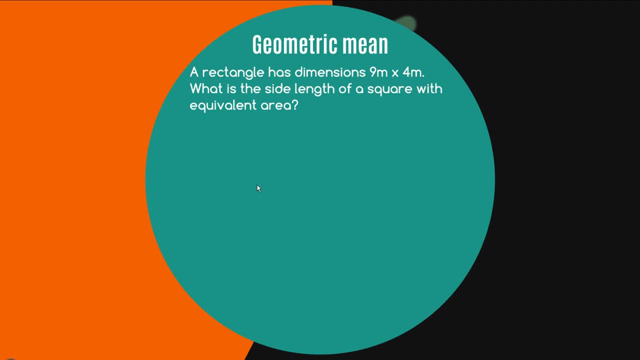 What's the side length of a square with equivalent area? So here's that rectangle 4 by 9.. It's 36 meters squared. So the question is, what square has an area of 36 meters squared? And you could probably tell me just from your own knowledge that the side length needs. 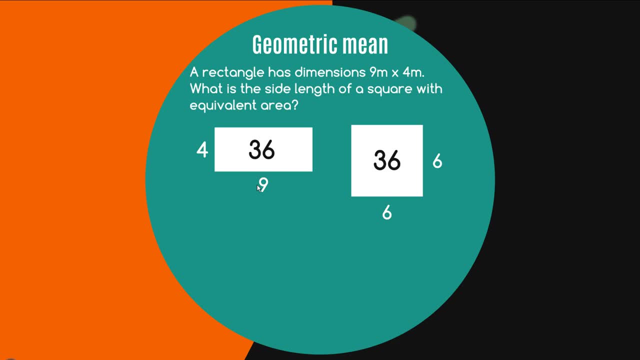 to be 6 meters. So in this case, 6 is actually going to be the geometric mean of 4 and 9.. But if you're to use the formula, the formula tells us to take the nth root of the product of the two observations. 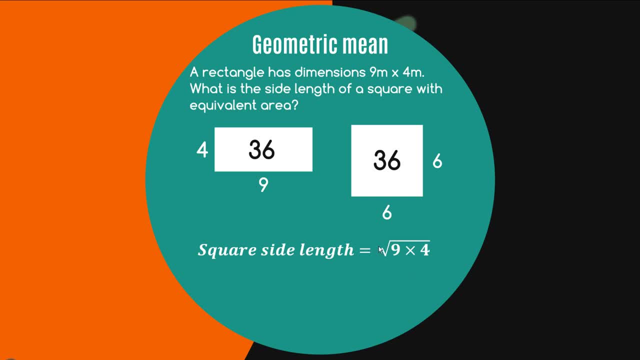 So 4 times 9.. We're going to multiply that together. We're then going to take the square root, because there's only two observations. So the nth root becomes the square root. The square root of 36 happens to be 6.. 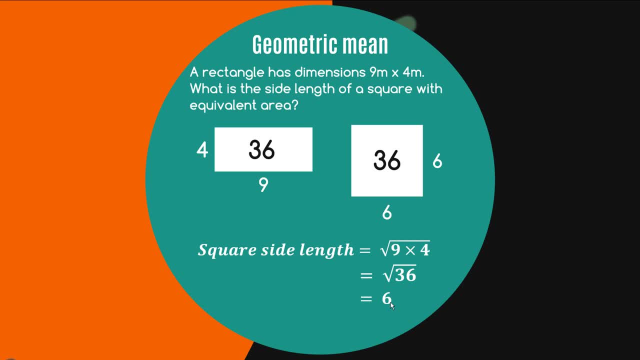 So that's where the geometric mean gets its name. But the applications extend well beyond geometry. My Tesla stocks gained 10% in year 1.. My theoretical Tesla stocks, that is 10% in year 2 and 30% in year 3.. 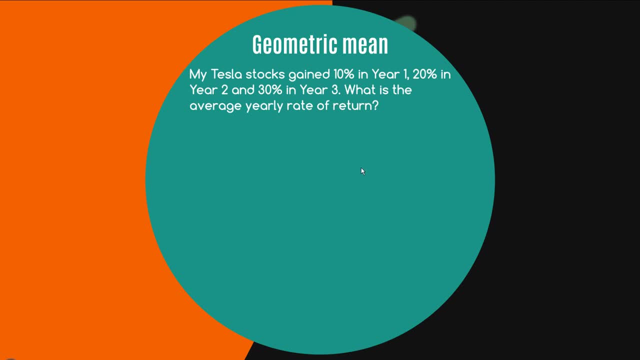 What's the average yearly rate of return? Now, this is a classic example of where geometric means come into the picture when you're dealing with rates of return. So here's a visualization of what's going on In year 0, we have $100, let's just say: 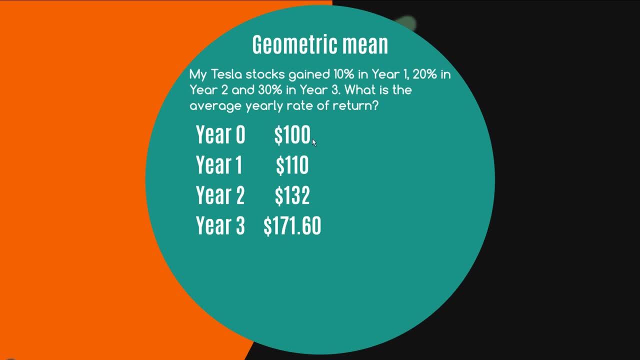 I've just put that in. It could have been any number of dollars here, but I've just chosen a nice round number. If I'm to gain 10% in that first year, that's going to take me 10%. That's going to take me to $110.. 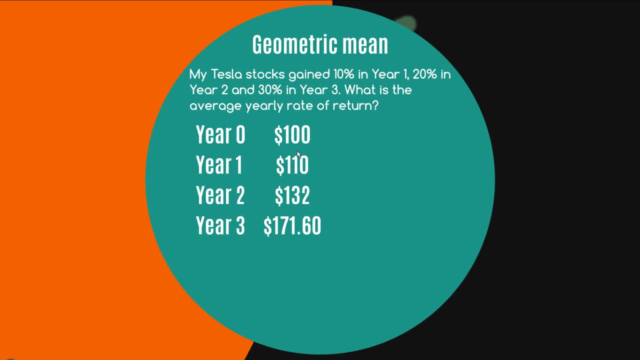 To gain 20% in that second year. well, it's 20% of 110, which gets added on, So that's going to get me to 132.. And then to add 30% on to the end of year 3 will get us to $171.60. 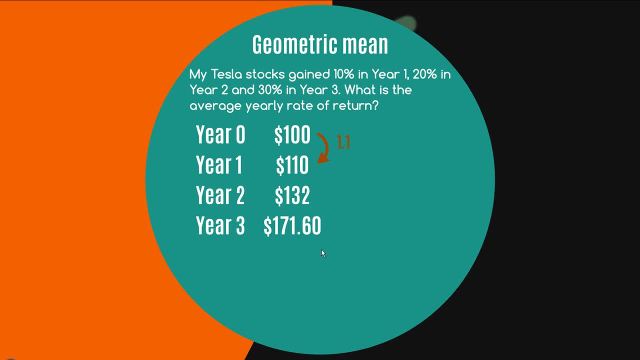 But essentially what's happened here is I've multiplied by 1.1 in the first instance, 1.2 in the second instance and 1.3 in the third. So you can see here that we have a changing yearly rate of return over the three years. 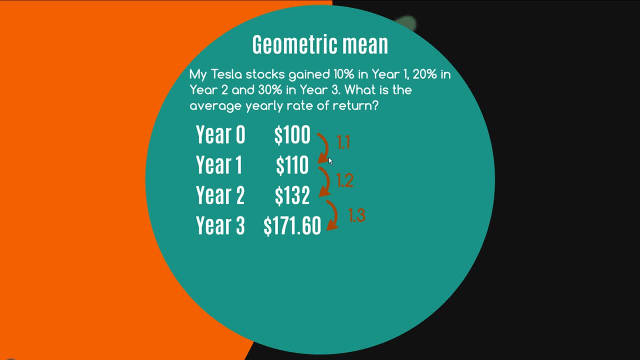 But what the question is asking is: can we find a yearly rate of return which is the same for each of these three years and still gets us to $171.60?? Now, the reason why this is a geometrical problem is that, if you think about a rectangular prism, 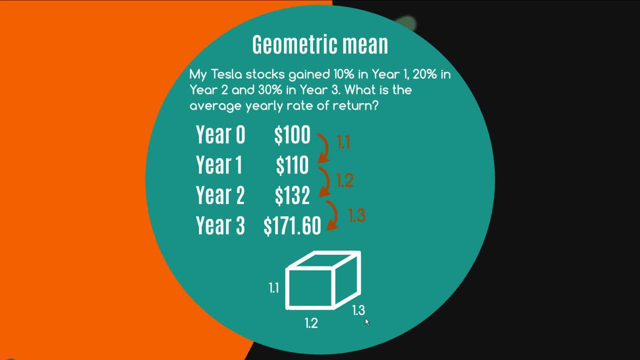 where the dimensions are 1.1,, 1.2, and 1.3.. Okay, respectively, we can ask what is the side length of a cube that has the same volume, And that's exactly the same question. So, even though this is a 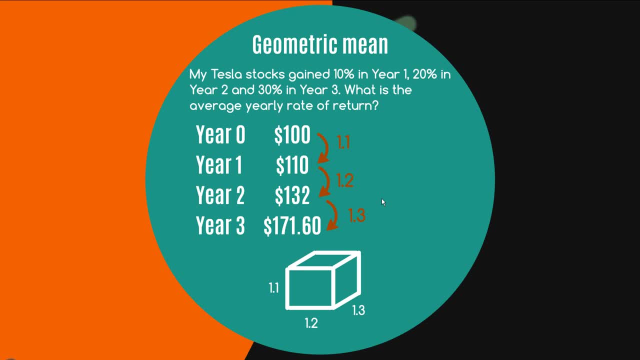 financial question. here there's this geometrical analogy, which is why this is a geometric mean. So how do we do this? Well, we know that multiplying these together, 1.1 times 1.2 times 1.3, gives us 1.716, so that is the. 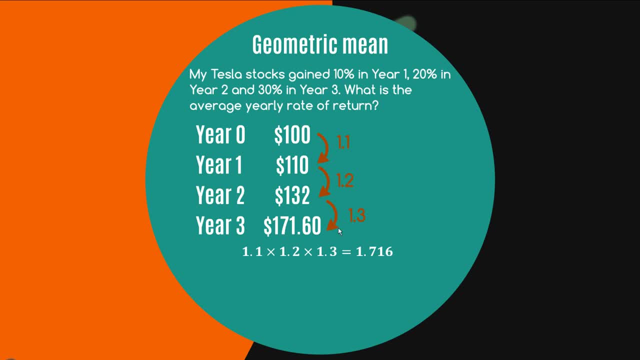 multiplier that gets us from Year 0 to Year 3.. You can see that represented here, which geometrically would be our volume right Now. what we have to do is take the cubed root of 1.716 and that will give us the effective average. 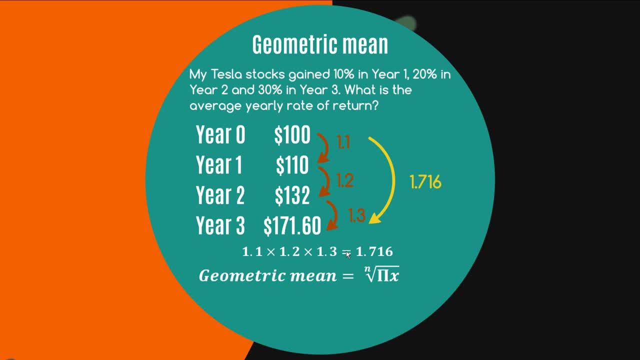 yearly rate of return. So the geometric mean- I've provided it again- here is the nth root of the product of x, That symbol, there is the Greek letter pi, which tells us to multiply all the elements of x. So it's going to be the cubed root of 1.716, which happens to be 1.1972. 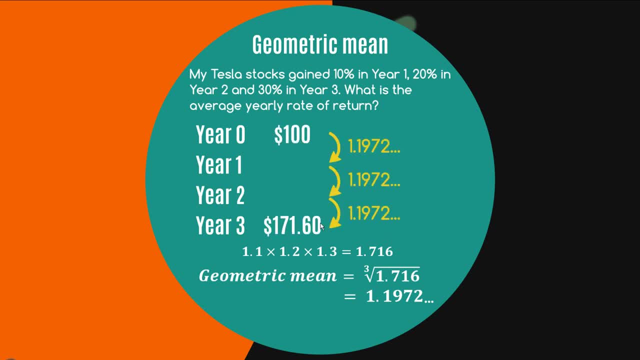 So, in other words, if you needed to get from $100 to $171.60 in three years, you could multiply by 1.1972. three times That means that our average yearly rate of return is 19.72%. You can lop off that first one point and have a look at just the increase, which is 19.72%. 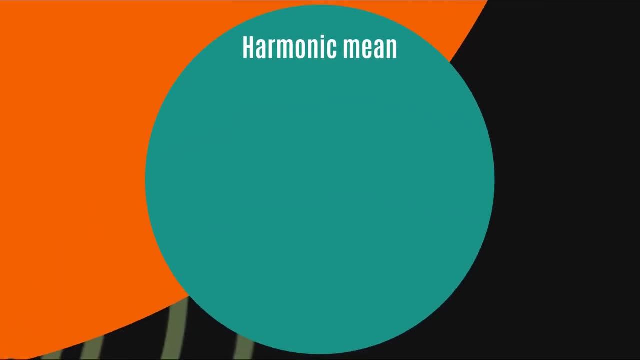 So let's have a look now at harmonic means. Now, harmonic means are used predominantly when you're dealing with rates, And one of the more common rates that you'll come across is that of speed, which is the rate of distance over time. 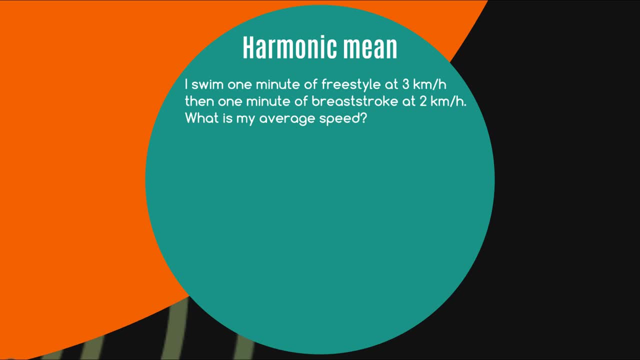 Here's a little example. If I say I swim one minute of freestyle at three kilometers an hour and then one minute of breaststroke at two kilometers an hour, What's my average speed? You'd be able to tell me that almost straight away: that my average speed is 2.5 kilometers an hour. 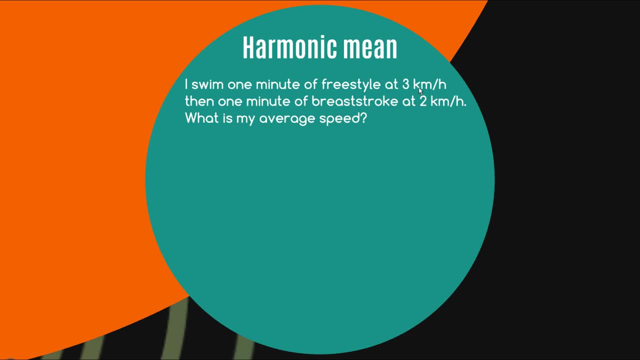 Why is that? Well, we can see the two speeds here and they're given as distances over time And we're averaging out across a single unit of time in each case, right? So when you've got a rate of distance over time and you're finding the average across fixed time, then the answer can be provided by finding the arithmetic mean. 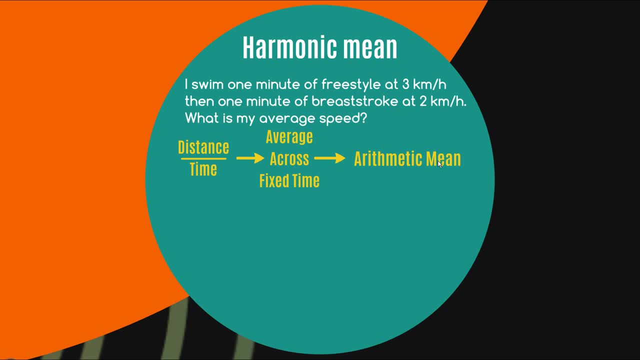 Just simply adding things up and dividing by n, which in this case is two. But what if I asked you this? I swim one lap of freestyle at three kilometers an hour and then one lap of breaststroke at two kilometers an hour. 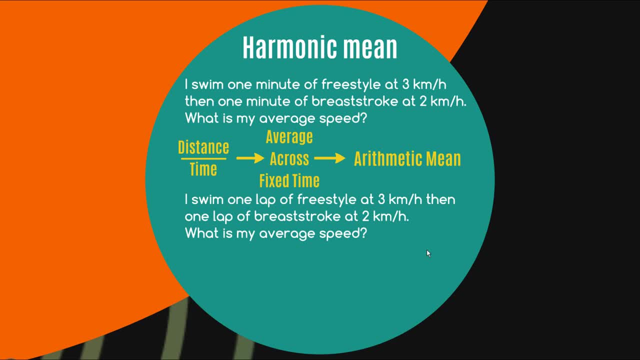 What's my average speed now? Well, this is no longer just an arithmetic mean, and hopefully you can see why. Clearly, my lap that I do at three kilometers an hour will be done faster than my lap that I do at two kilometers an hour. 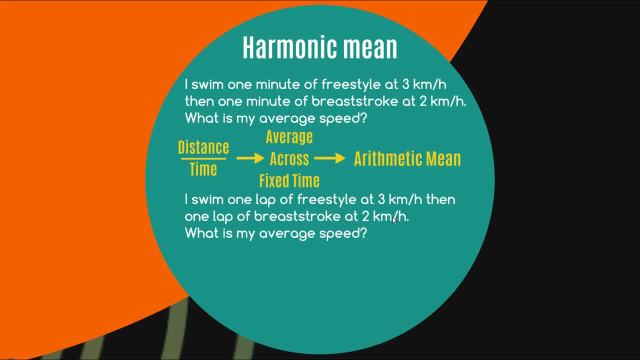 So if you look at the total time I'm spending swimming here, I'm spending more time swimming at two kilometers an hour than I am swimming at three kilometers an hour. So the average speed is no longer going to be just 2.5. 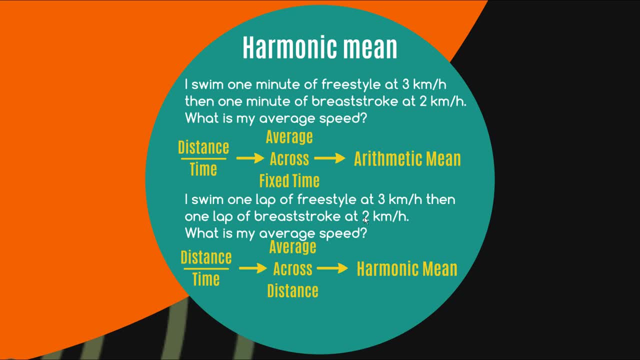 kilometers, It's going to have to be the harmonic mean of both 2 and 3.. So whenever you have a rate like this distance over time, if you're trying to find the average across a fixed distance, which is the numerator of the rate, the 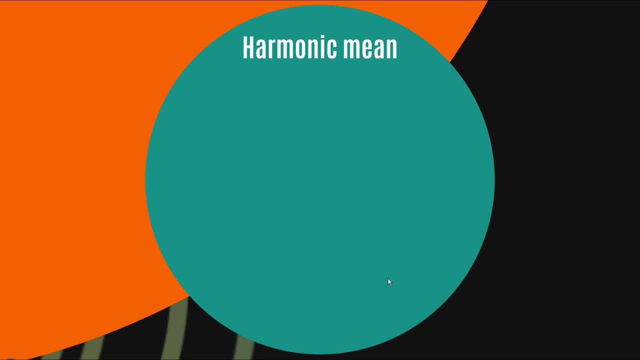 solution will be a harmonic mean. So let's indeed find out how that gets calculated. Now I'm just repeating that harmonic mean question up here where we've got a lap of freestyle and a lap of breaststroke. So here's the formula to: 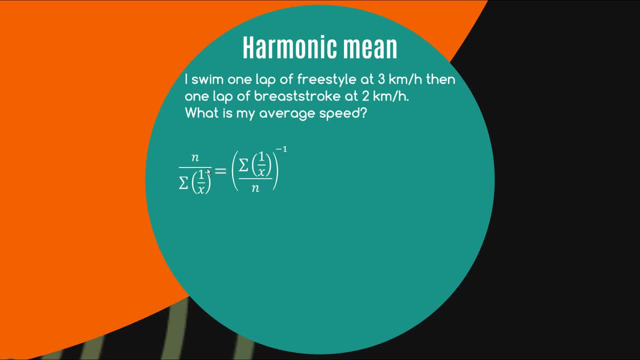 find the harmonic mean. It's n divided by the sum of 1 on x. but I've reconfigured it here just to show you what really is happening. here We have the sum of 1 on x divided by n, so the average of the inverted observations, And then taking 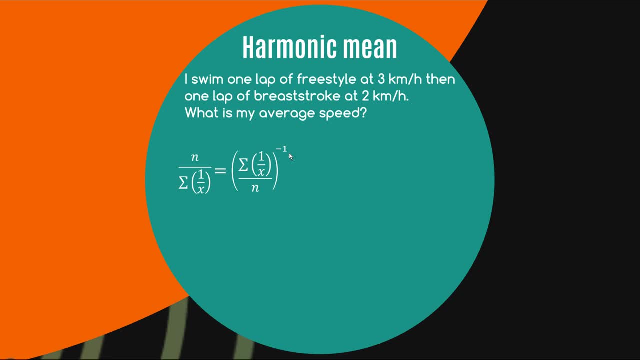 the inverse of that. so it's almost like we flip it over, find the average and then flip it back. And that kind of makes sense, right, because we need to find the average across this fixed distance. So So we need to flip these rates so they're no longer distance over time, but rather time. 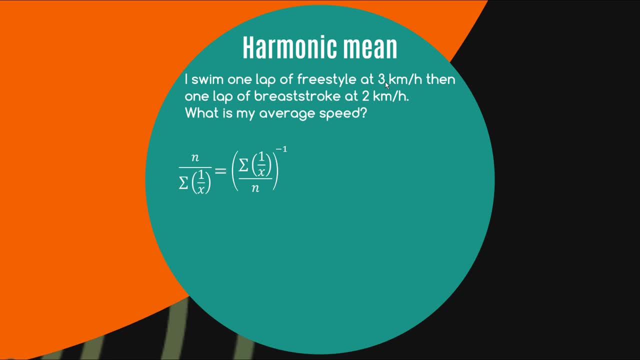 over distance. And then, of course, we need to flip it back once we find that average. So here it is, using that formula, instead of three plus two divided by two, we now have one on three plus one on two divided by two, and then we invert that. 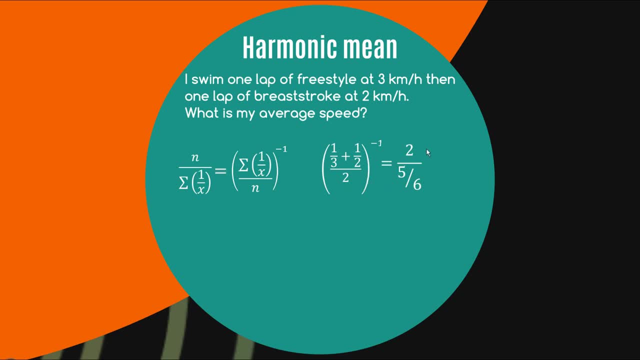 And so, using a little bit of algebra here, which hopefully you're up to, it's going to be two divided by five on six, which turns out to be 2.4.. So my average speed here is 2.4 kilometers per hour. 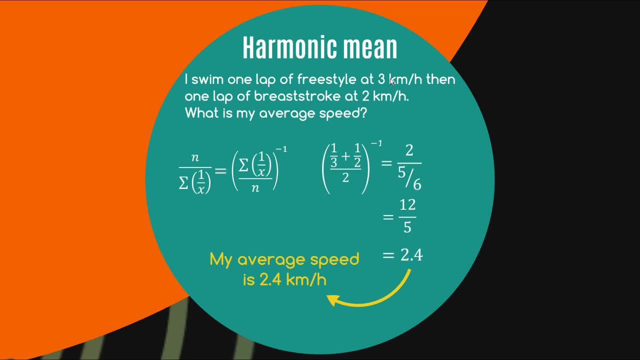 And you'll notice that it is slightly closer to two than it is to three. That's kind of what we expected, right? Because we're swimming at two kilometers an hour for slightly longer than we're swimming at three kilometers an hour because of the fixed distance. 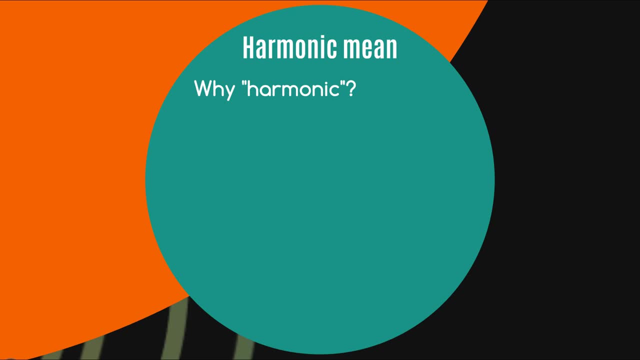 Now, if you're interested in knowing why it's called a harmonic mean, I've just prepared a little kind of aside here just in case you wanted to know, for anyone that's interested. It indeed comes from the word harmony, from music, And I'll try to do this quite quickly. but the idea is that whenever you have a particular 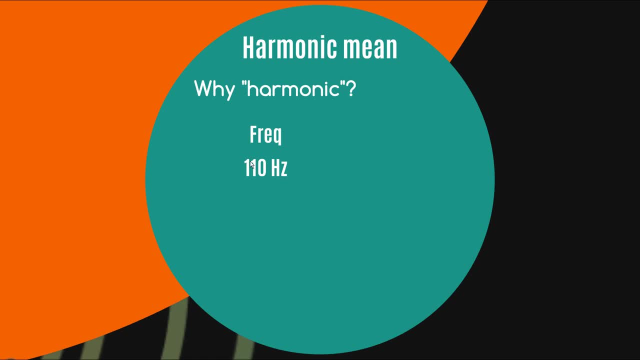 musical note. let's say that note A, let's just say this particular A has a frequency which is 110 Hertz. Not only when I hit that string does this frequency sound wave get emanated, but there are all these other harmonic overtones that also emanate from that particular strike of 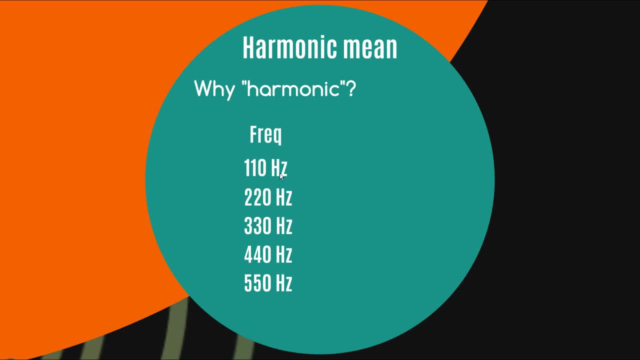 that string. So I'll get 110 Hertz as the frequency that comes out, but I'll also get 220, a little bit of 330, a little bit less of 440, et cetera, et cetera. 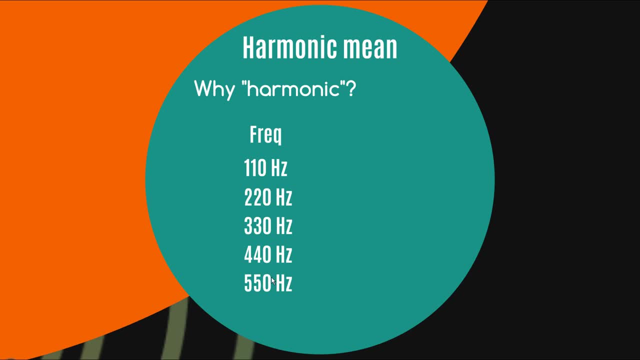 And these are called harmonic overtones. Now we don't need to get into the musicality of all this, But appreciate. if you've done any science, you remember that wavelength is actually proportional to the inverse of these frequencies. So if you call the wavelength one for this frequency, 110 Hertz, the wavelength for 220. 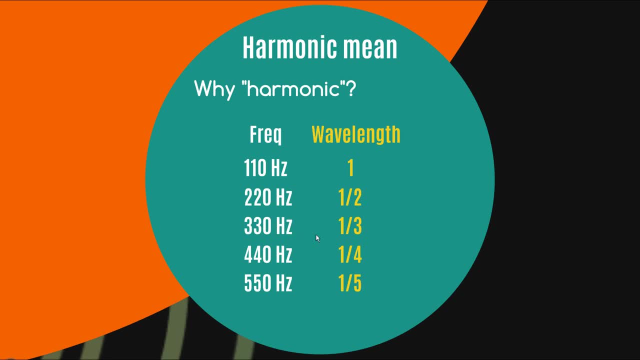 Hertz will be half of that And the wavelength of 330 Hertz will be a third of the original wavelength. So what happens is that these wavelengths are in fact in a harmonic series, so that the harmonic mean, So the harmonic mean of this wavelength one on two and this wavelength one on four. 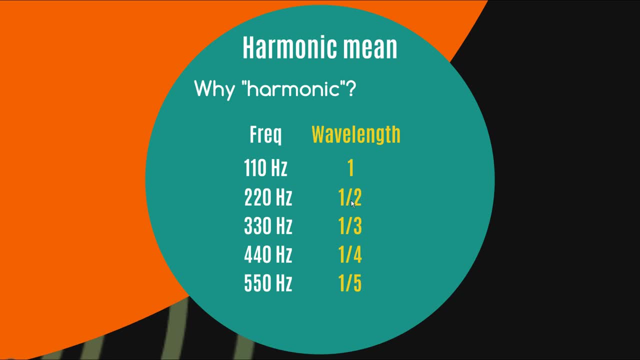 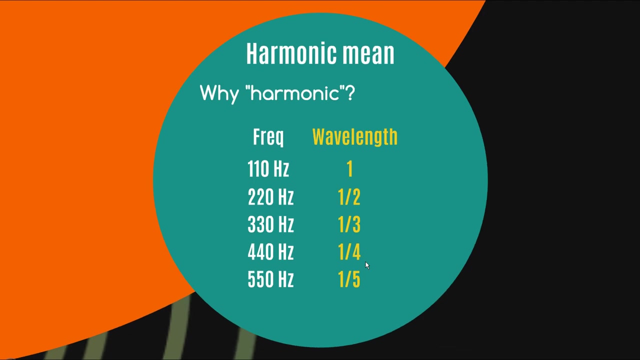 is actually one on three. So you can see, it's because of this whole inverting that happens between frequency and wavelength that to find the average of two particular wavelengths you need to find the harmonic average or the harmonic mean. Now I'm going to leave you with a challenge question which I'm not going to answer myself. 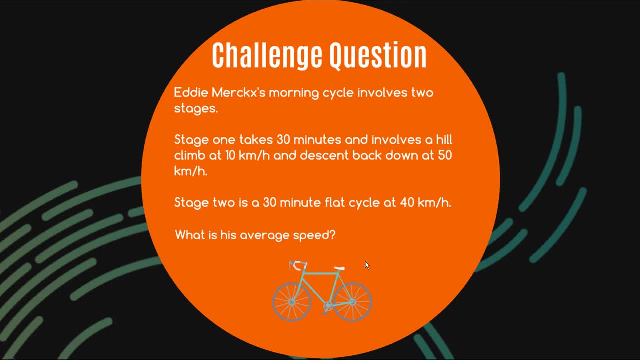 but I'm hoping you will provide your answers in the comments. But, as you can see, it's all about Eddie Merckx and his morning cycle, So I'll leave that with you. My name is Justin Zeltser from zstatisticscom.